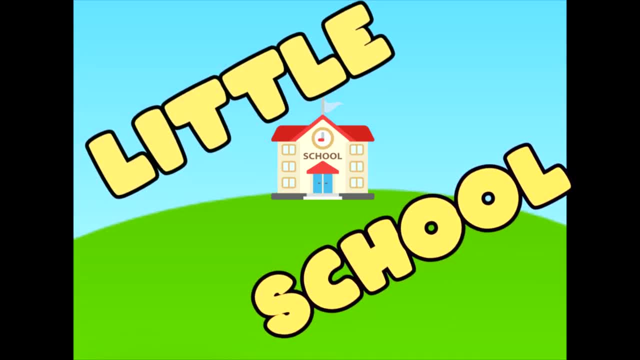 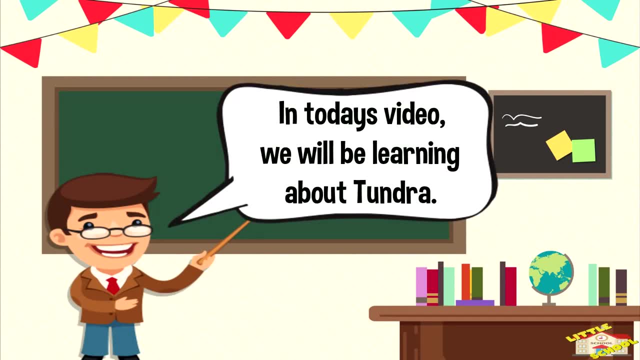 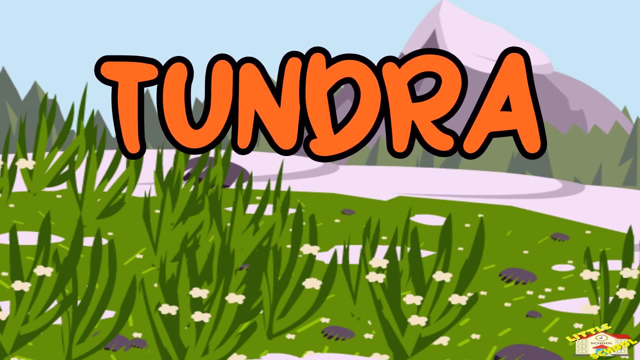 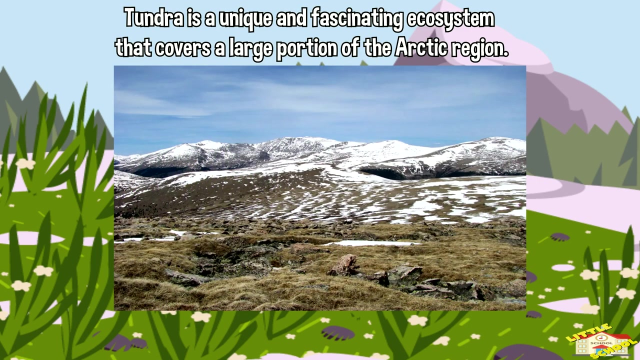 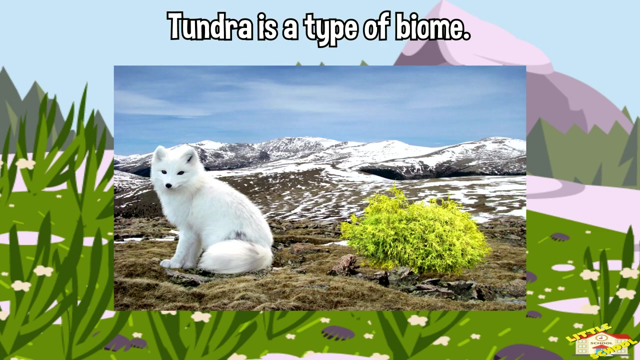 Hey kids, In today's video we'll be learning about tundra. Are you ready? Let's begin. Tundra is a unique and fascinating ecosystem that covers a large portion of the Arctic region. Tundra is a type of biome, which means it is a large area of land that has a specific 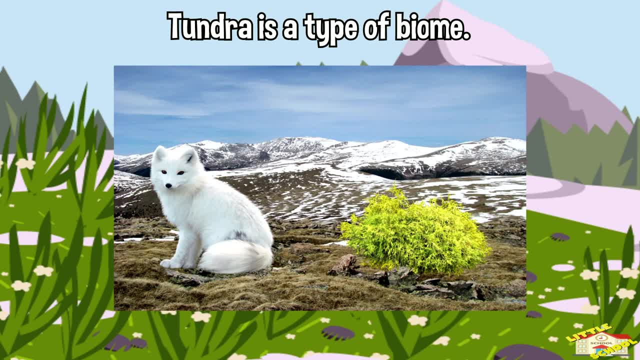 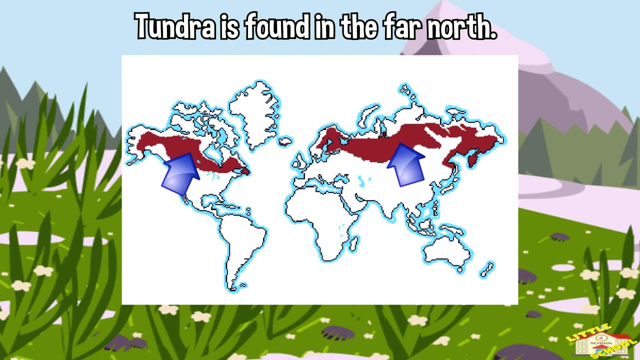 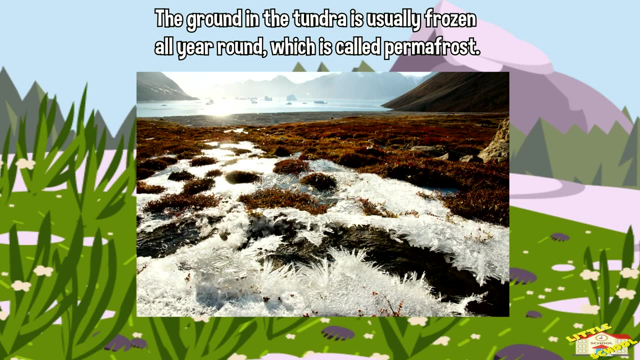 climate and supports specific types of plants and animals. Tundra is found in the far north, where it is very cold and there is little precipitation. The ground in the tundra is usually frozen all year round, which is called permafrost. Because of the permafrost, 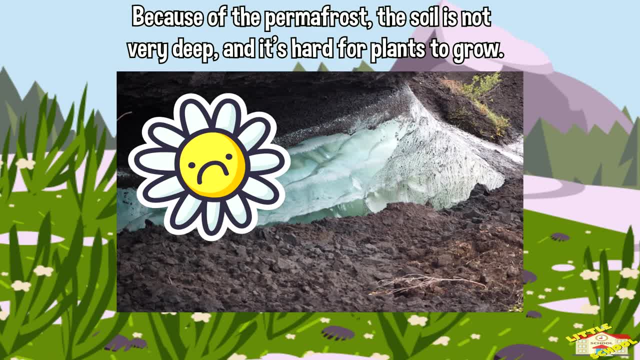 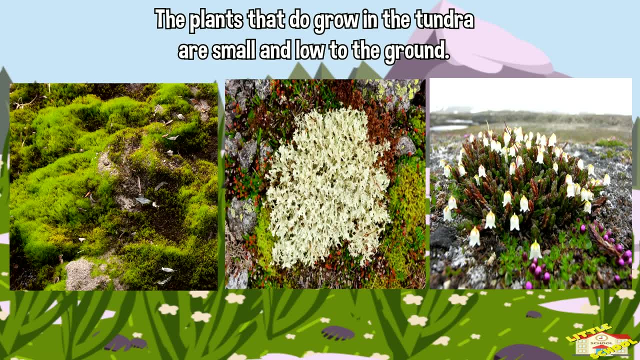 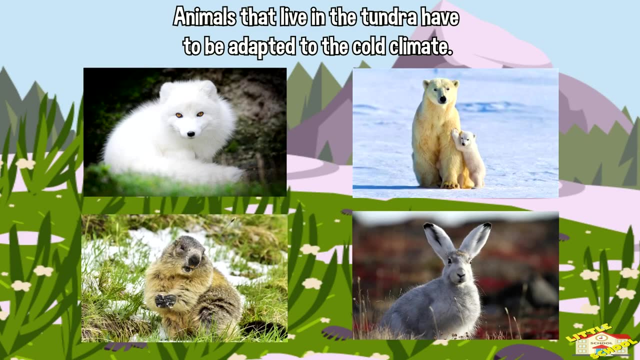 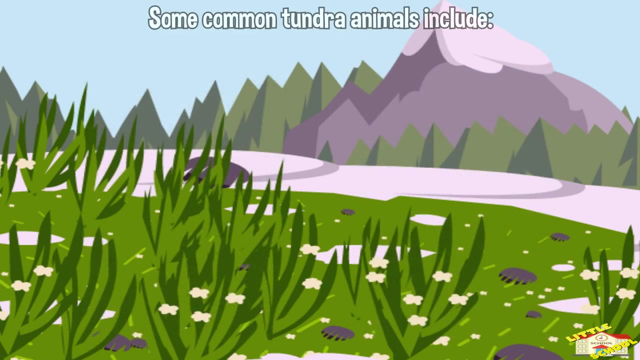 the soil is not very deep and it's hard for plants to grow. The plants that do grow in the tundra are small and low to the ground, such as mosses, lichens and shrubs. Animals that live in the tundra have to be adapted to the cold climate. Some common tundra animals include caribou. 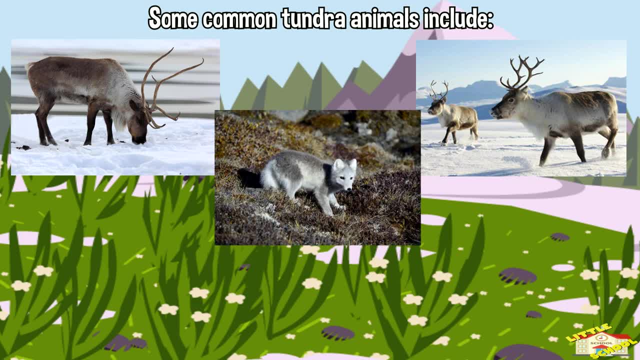 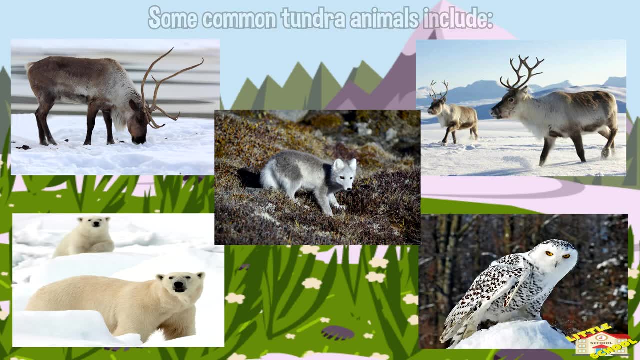 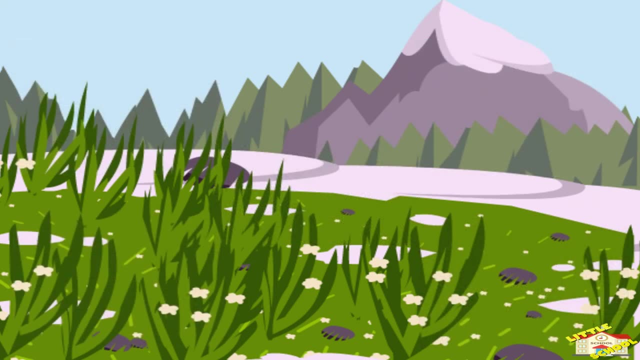 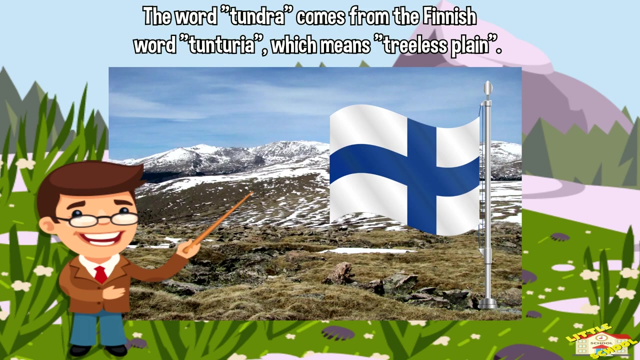 reindeer, arctic foxes, polar bears and snowy owls. These animals have thick fur or feathers to keep them warm. Now here are fun facts about tundra. The word tundra comes from the Finnish word tunturia, which means treeless plain. 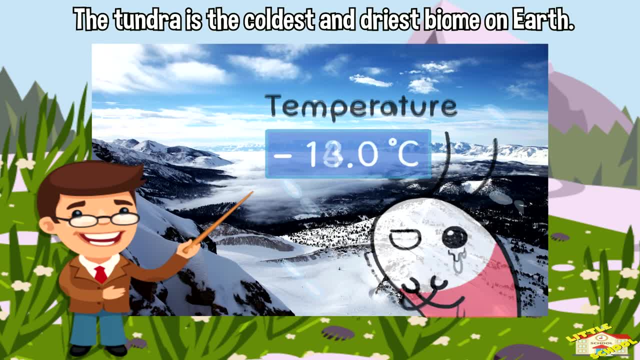 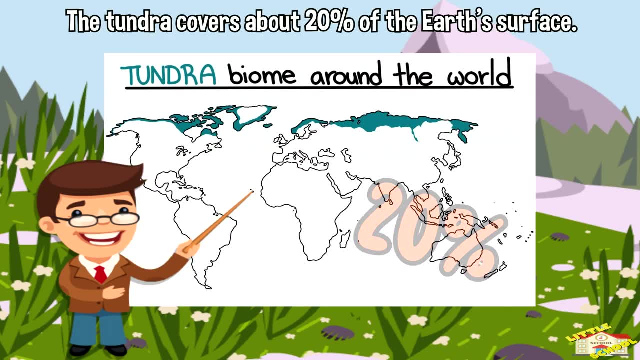 The tundra is the coldest and driest biome on earth. The tundra is the coldest and driest biome on earth. The tundra is busy on every summer, with temperatures often below freezing and very little precipitation. The tundra covers about 20% of the earth's surface. 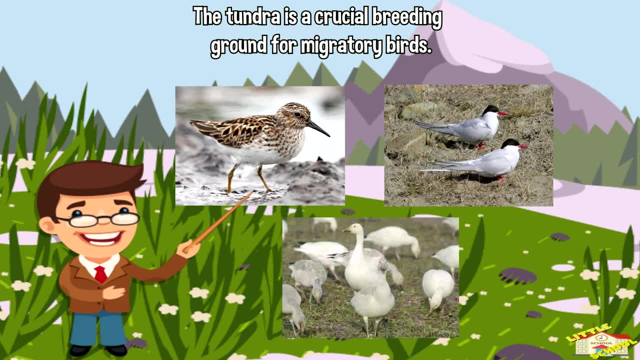 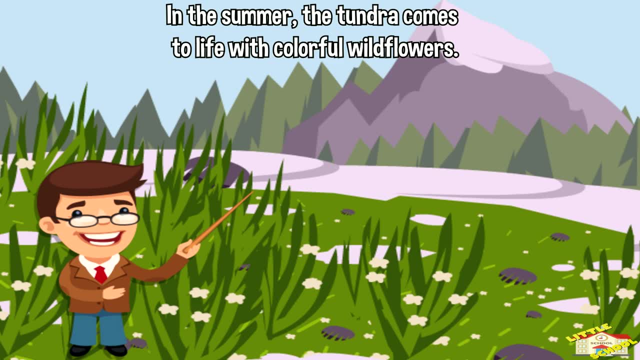 The tundra is a crucial breeding ground for migratory birds such as sandpipers, terns and snow geese. In the summer, the tundra comes to life with colorful wildflowers such as the arctic poppy and sacksey kami.